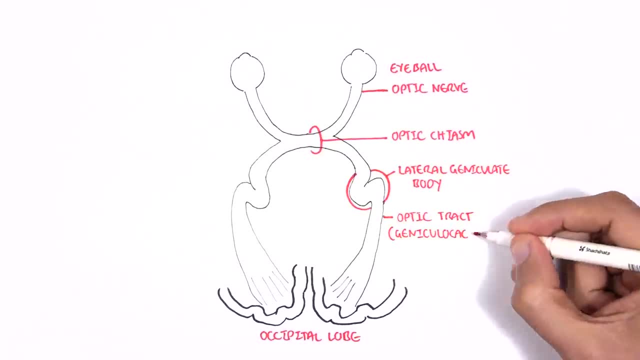 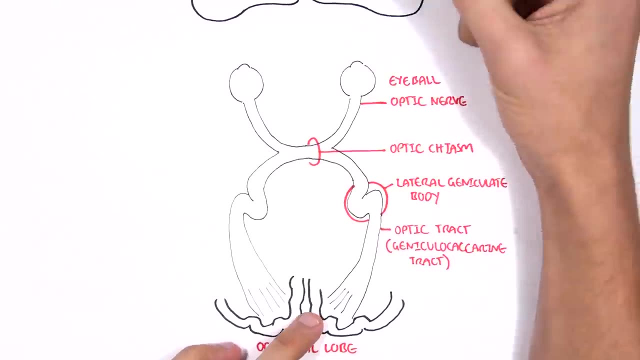 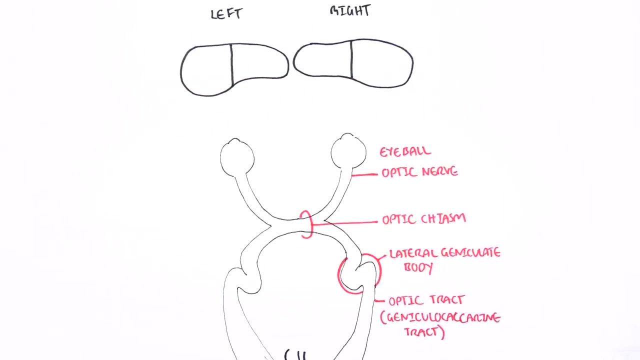 geniculate body and optic tract, also known as a genicocacrine tract. Here are our visual fields. We are looking at this whole visual pathway, you know, from the top. So the blue nerve on the left side here will pick up the left nasal field and will carry. 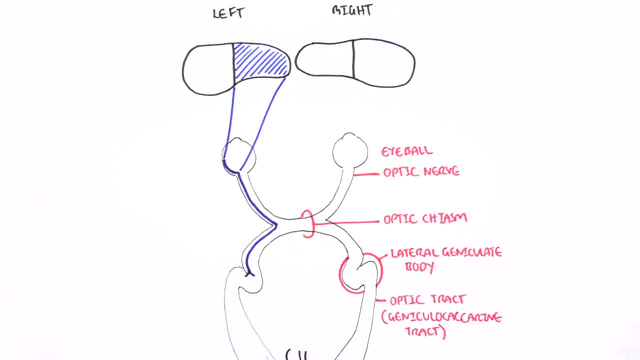 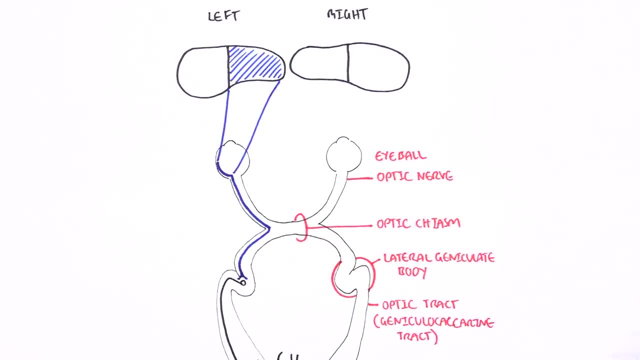 this visual information to the lateral geniculate body, where it will synapse with a another nerve, and this other nerve will then carry this information to the occipital lobe. The blue nerve on the right eyeball here will capture images from the right temporal field. 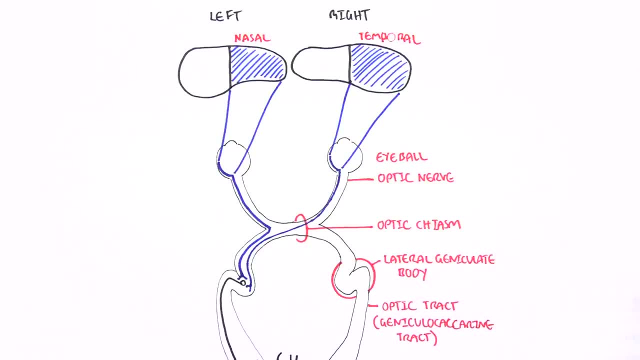 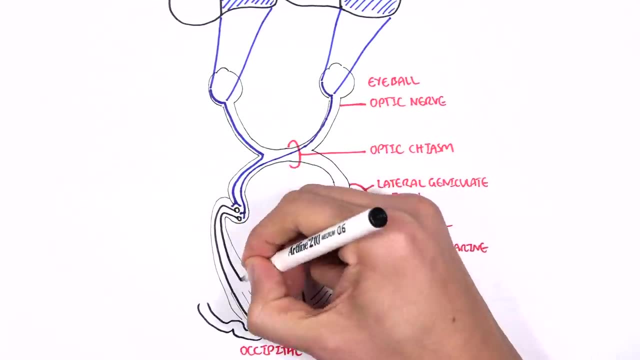 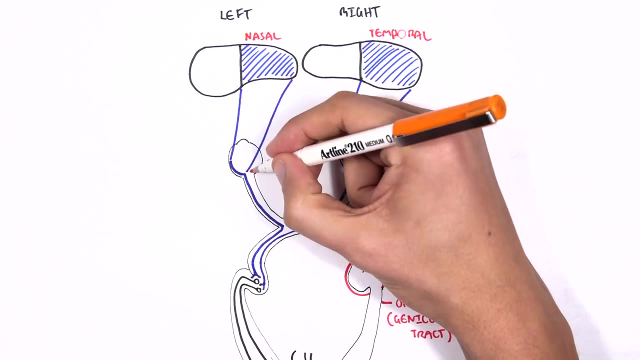 and will carry this information down the optic nerve and will cross over at the optic chiasm and synapse with the neurons of the left lateral geniculate body. The nerves will then carry the information to the occipital lobe. This orange optic nerve on the left eyeball here will capture images from the left temporal. 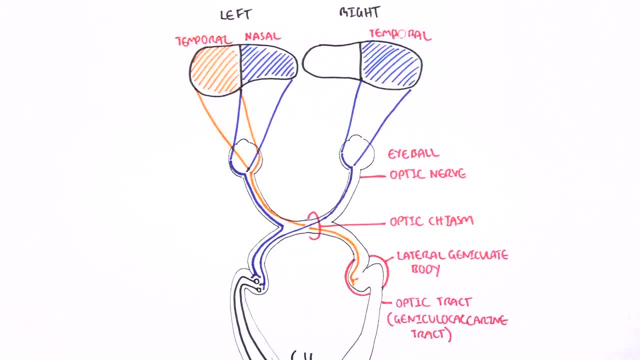 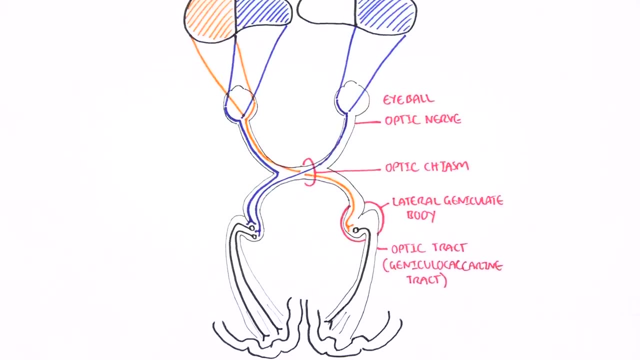 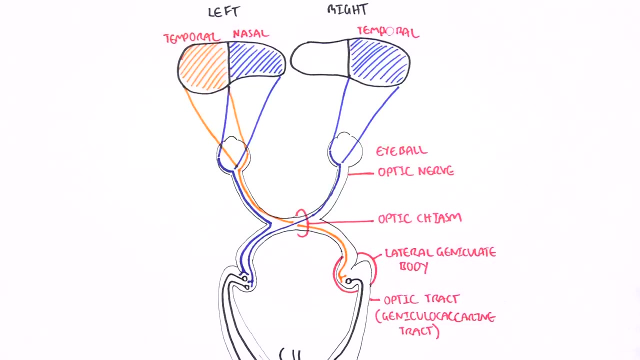 visual field and cross over at the optic chiasm and synapse at the right lateral geniculate body, where it will relay the information to the optic tract, which then will bring it to the occipital lobe. Now, similarly, the orange optic nerve of the right eye will capture the image from the 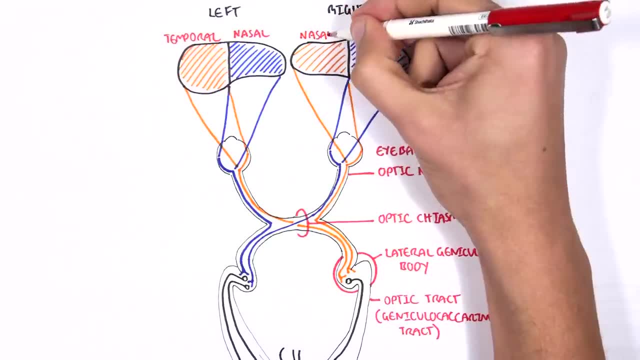 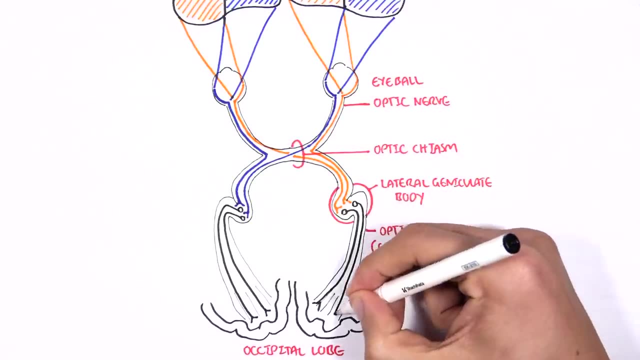 right. It will not cross over but will relay this information down to the lateral geniculate body and then it will synapse with other nerves along the optic tract and then down to the occipital lobe. I hope this pathway makes sense. 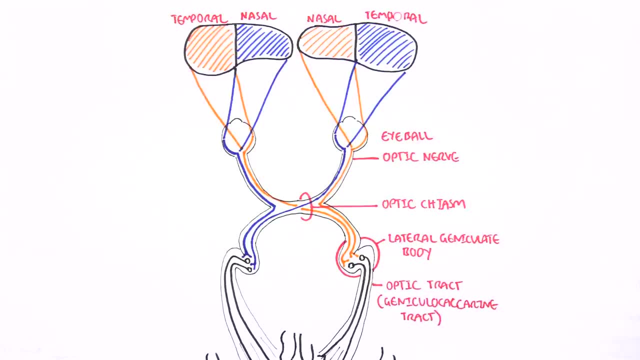 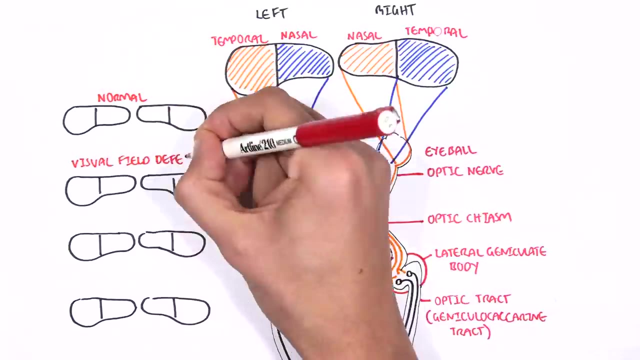 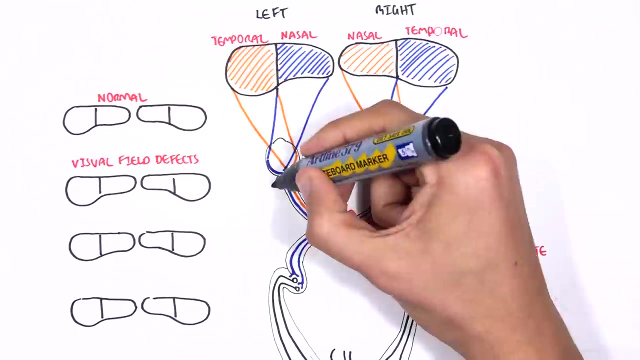 Now that we have an overview or an understanding of the visual pathway, what happens to our vision if we have lesions occurring along these different pathways? Let's take a look. So let us have a look and compare normal to defects in visual fields. If a lesion were to occur on the left optic nerve A, what happens is that the orange 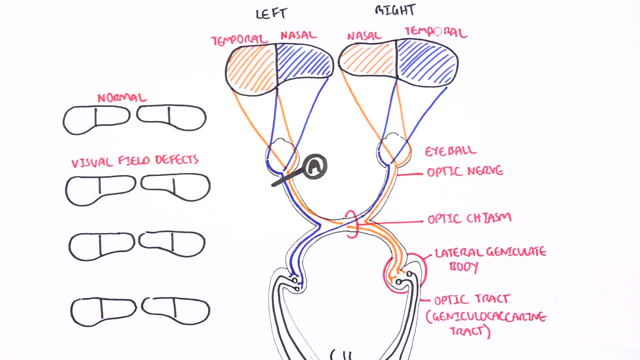 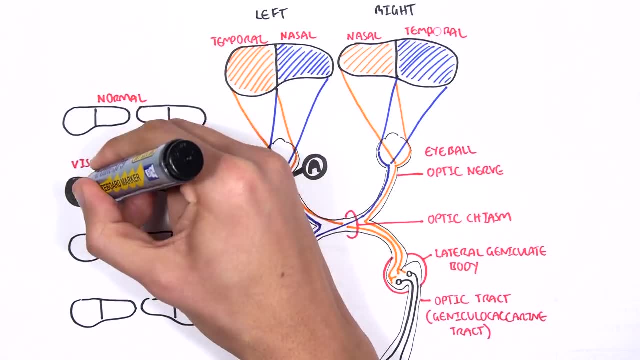 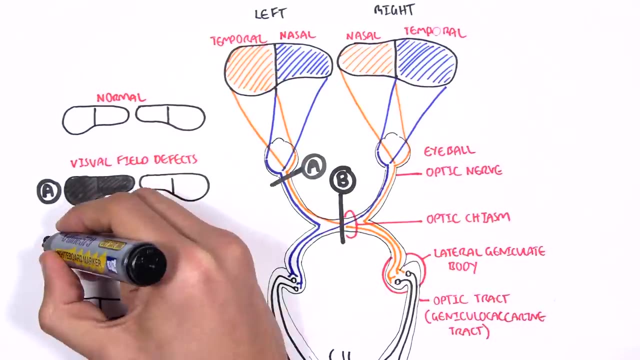 and blue optic nerve on the left side cannot even bring the information down, and so we get blindness in the left eye. This is called left anopia. If a lesion occurs along the optic chiasm here in B and this can be due to a pituitary, 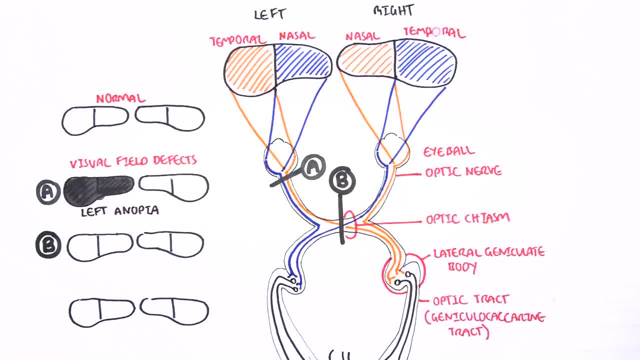 tumor. well, the nerves that cross over that normally captures images on the temporal visual fields cannot send this information, and so we get blindness in the temporal visual fields from both the left and the right anopia. This is called left anopia- This is called left anopia. 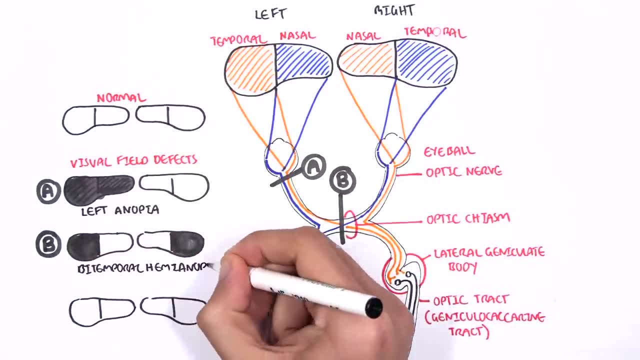 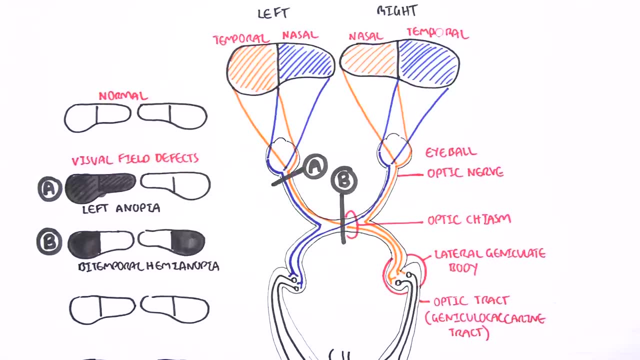 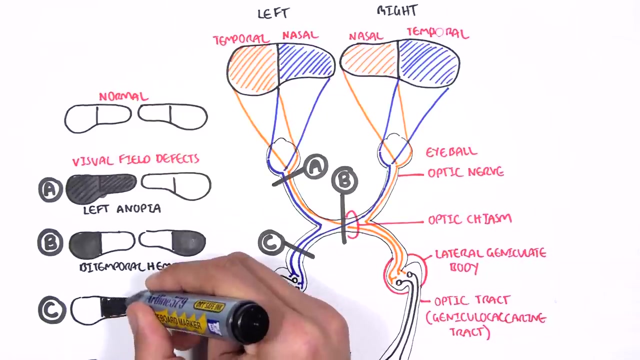 If a lesion occurs here after the optic chiasm, we get loss of the visual fields that these blue nerves carried, which means we get loss of vision on the left nasal field and the right temporal field. This is called right homonymous anopia. 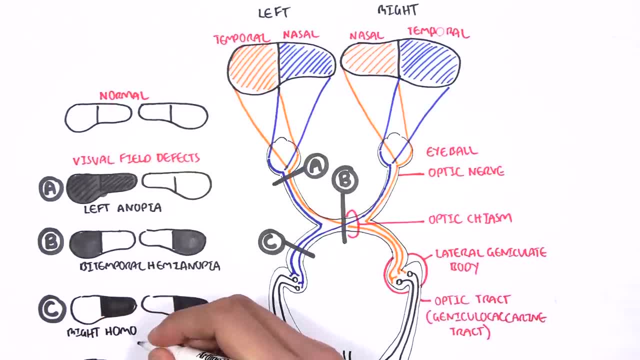 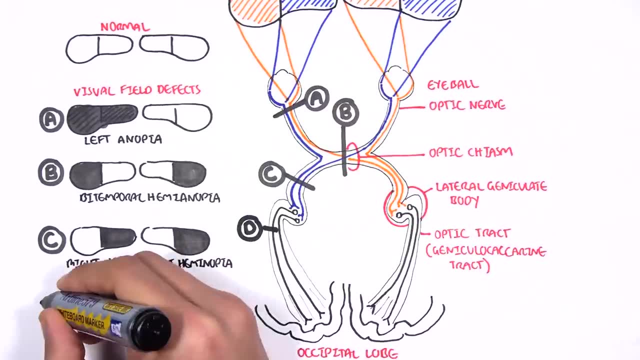 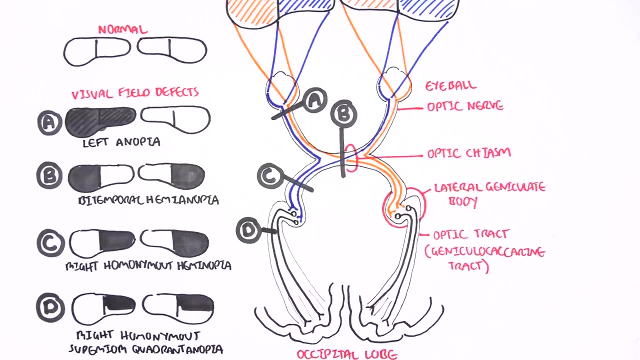 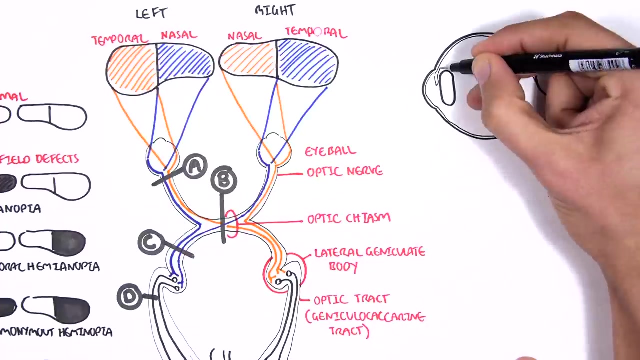 If a lesion occurs here after the optic chiasm, we get loss of the visual fields that these blue units carry. This is called up to white anopia. If a lesion occurs on one of these nerve tract bundles, it will cause the condition. 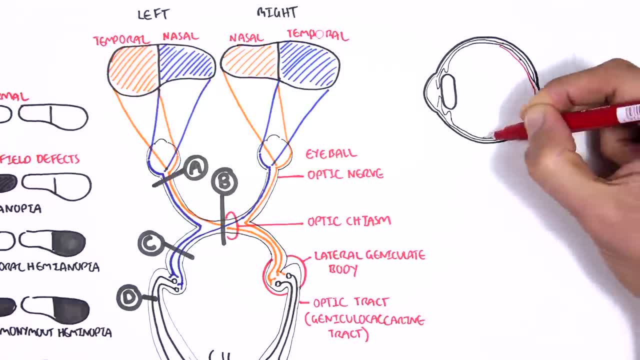 Let us cut a cross section of the eyeball and learn some important structures. So here is the optic disc where the optic nerve and vessels of the eyeball pass through. Here is an area within the eyeball at the very back, called the macula. 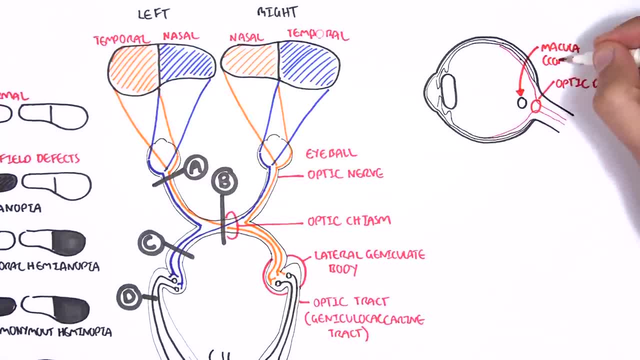 Now, the macula contains what's known as a fovea, which is an area where a lot of pigmented cells are called cones, And these pigmented cells of the retina, these guys allow for high resolution. So when we damage the macula, we get loss of central vision.